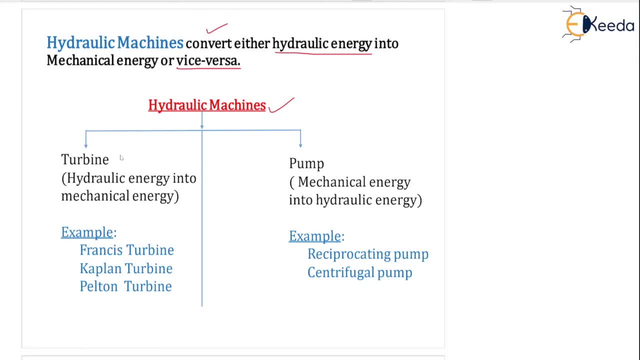 energy. So this mechanical energy will be developed into electrical energy, Correct. So hydraulic energy in the turbine, your hydraulic energy, will be converted into mechanical energy and this mechanical energy will be again developed into electrical energy. Correct, and that is how we are getting electricity. 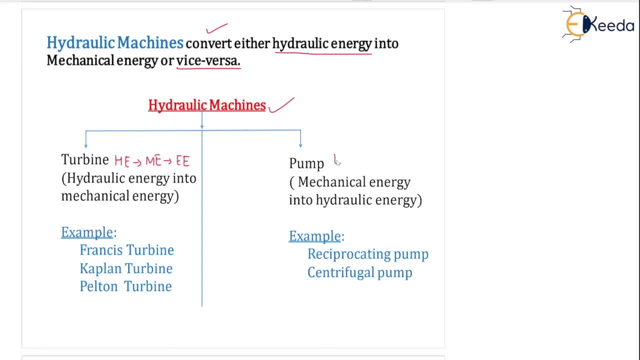 But in the pump, first of all, we are supplying the electrical energy. With the help of this, electrical energy is developed into mechanical energy, and this mechanical energy is then converted to hydraulic energy. Correct, So this is the chain of transformation of energy. But what we are going to in this? 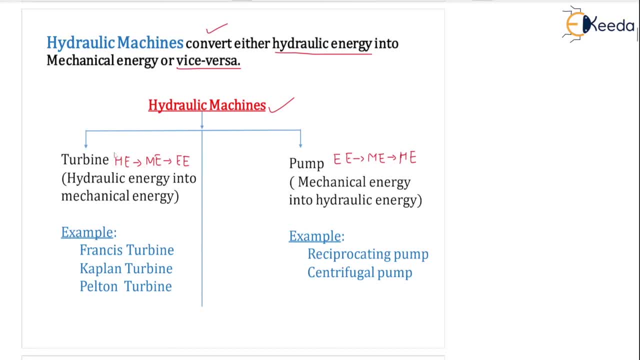 chapter is we are going to see the conversion of your hydraulic energy into mechanical energy. The electrical part is not in our syllabus. Same way here: mechanical energy to hydraulic energy. Okay, So what are the example of turbine here? Turbine example you can see. 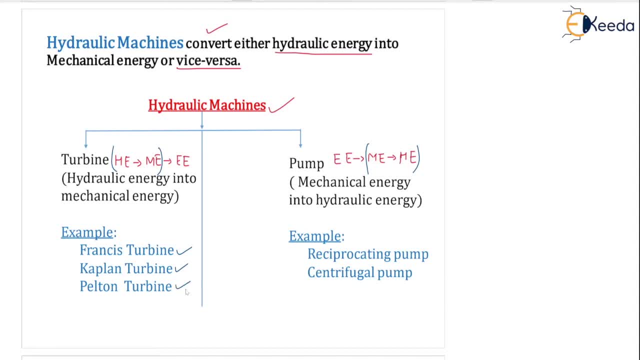 the Francis turbine, the Kaplan turbine and Pelton turbine. Out of these three, Pelton turbine is very, very important. Example of pump. you can see a reciprocating pump. We are also having rotary pump and centrifugal pump. Some more details about the hydraulic machine. So this is a chapter very, very important because this: 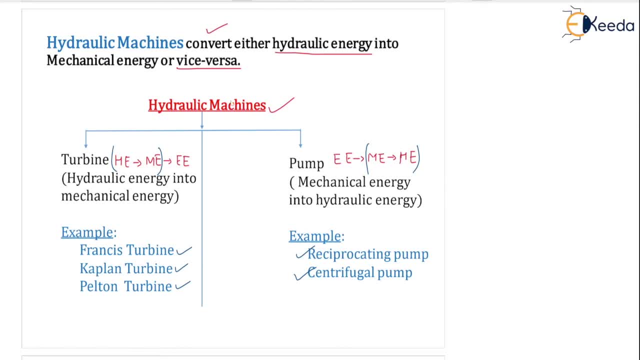 is giving you the structure of the entire hydraulic machine. So first of all we are going to see the hydraulic machines definition we have seen right now, correct hydraulic machine definition, and then we are going to see about the turbine, then Francis turbine, Kaplan, Pelton, it turbine. We are going to see one by one, Then we move to pump and then we will see. 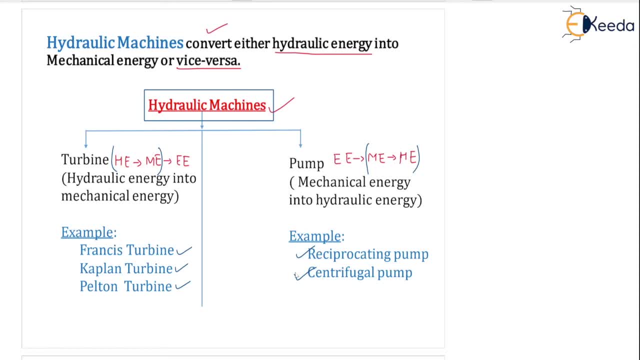 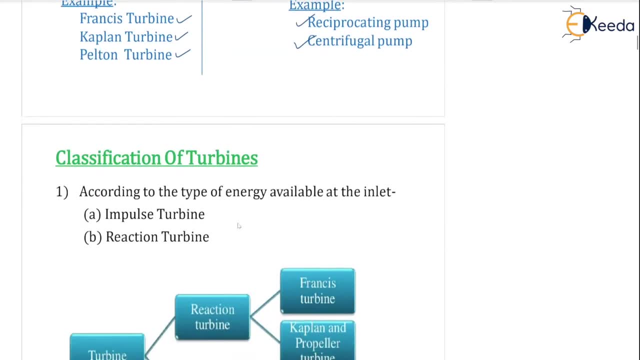 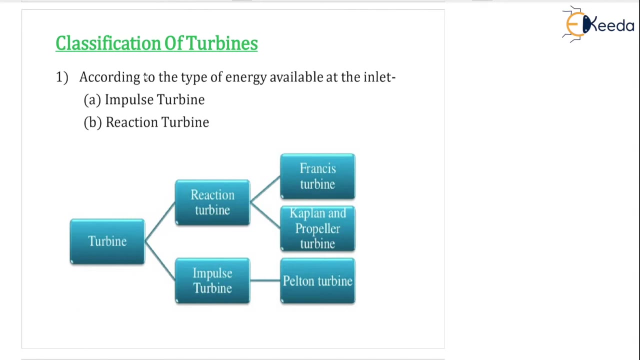 the specific speed of pumps. Okay, and then in the last we're going to see velocity triangle. So let us start with the turbine. Classification of turbine first of all. So hydraulic machines definition. we have seen under that we are having turbine and pumps. So now we are going to complete. first, 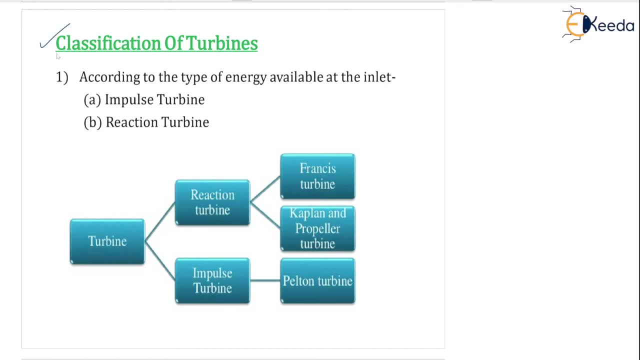 turbine part. So classification of turbine is the next topic here. So according to the type of energy, how we can classify the turbine. There are many parameters by which we can classify the turbine. Number one: according to the type of energy. type of energy available at the inlet. correct available at the inlet. 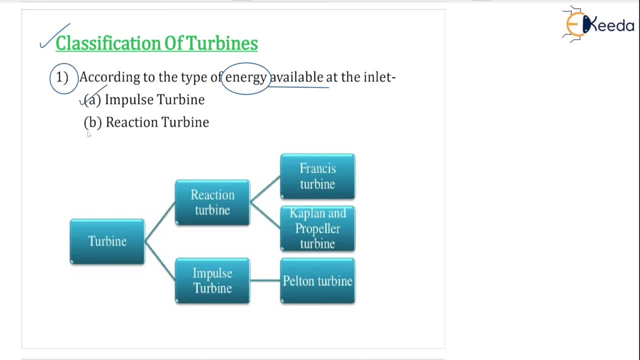 So out of this classification we are having impulse turbine and reaction turbine. So we are going to define definitely what is impulse and what is reaction turbine As of now- you can see the diagram here. Turbine is classified into reaction turbine and impulse turbine. Already it is written here. 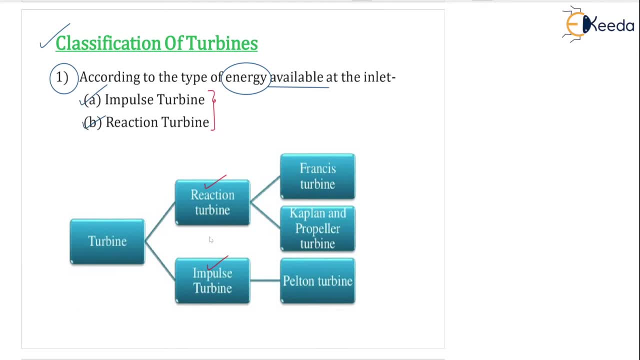 impulse and reaction turbine. Impulse turbine- name is your, Pelton turbine is an example, and reaction turbine is Francis turbine. Kaplan and Proffiler turbine comes under the reaction turbine. Francis is reaction turbine whereas Pelton is the impulse turbine. correct So three turbines we have mentioned in the list, correct So Kaplan. 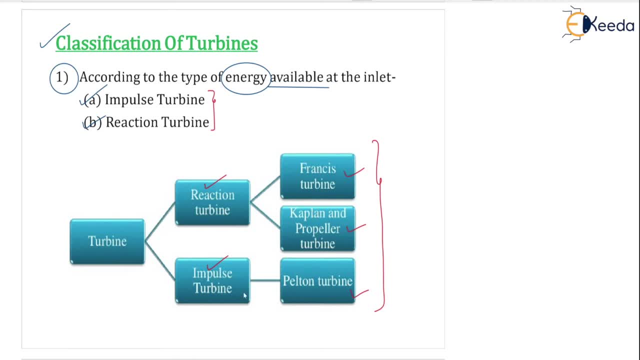 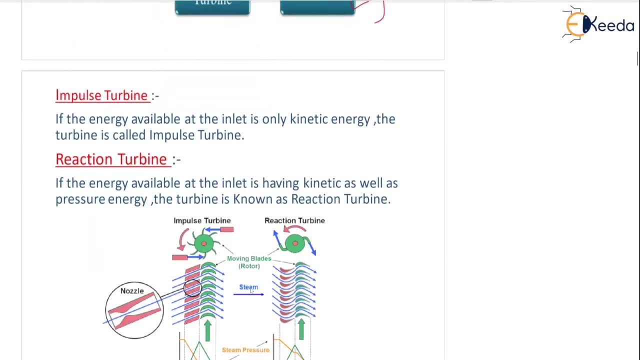 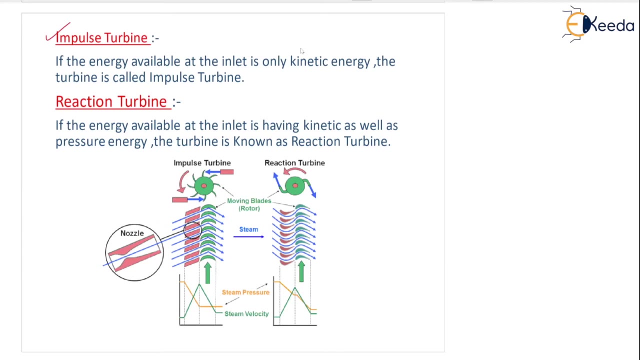 and Francis comes under reaction turbine. Pelton is impulse turbine. Now we are going to see in detail what is impulse and what is reaction turbine. Look at the complete detail about the impulse turbine. If the energy available at the inlet is only kinetic energy- very, very important. If the energy available 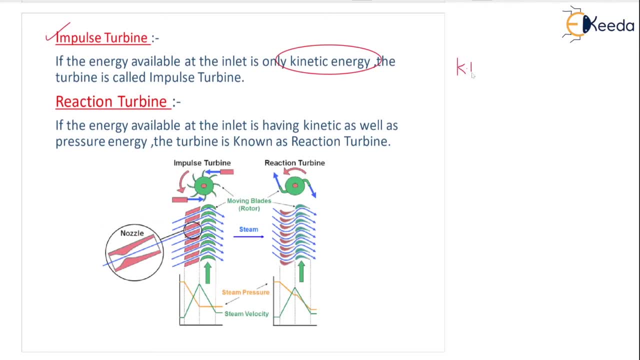 at the inlet is only kinetic energy, correct. The turbine is called as impulse turbine. The turbine is called as impulse turbine. So you know that if you talk about the total head, we are having pressure head p by rho g, correct, plus velocity at v square by 2g, plus z datum head. 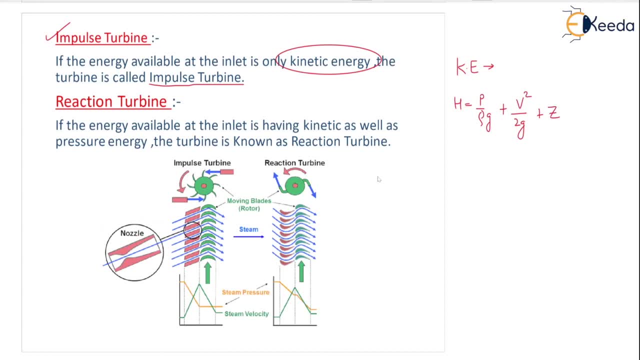 So if the energy available at the inlet is only kinetic energy, that is, kinetic head, the turbine is called as impulse turbine, Reaction turbine. if the energy available at the inlet is having kinetic energy as well as pressure energy, the turbine is known as reaction turbine. 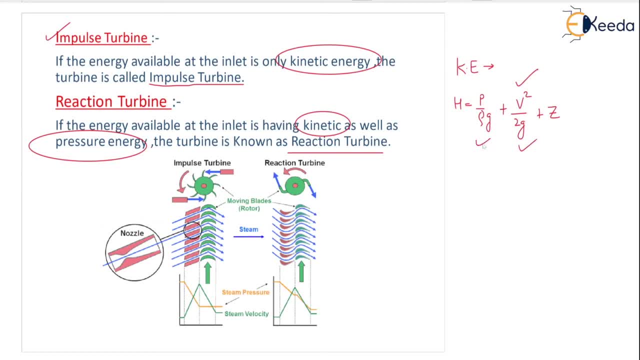 So along with the velocity head we are also having pressure head. Then the turbine is known as your reaction turbine. In the first case it is known as impulse turbine, IT. Okay, Now you can see the example of here. some diagram is given: impulse turbine and 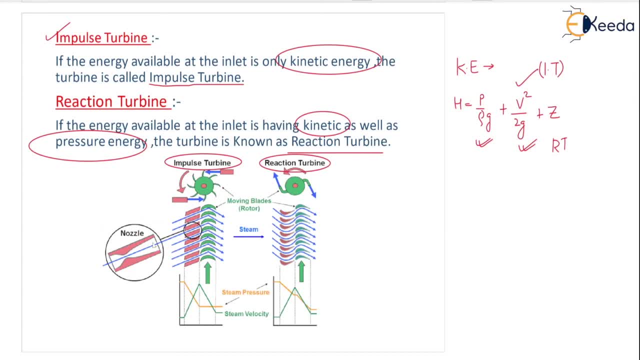 reaction turbine. Okay, What is the difference? Please see here. So from the nozzle the water is sprayed, the fluid is coming out of the nozzle And this nozzle is, you can see it is convergent divergent nozzle. And this nozzle is, you can see it is convergent divergent. 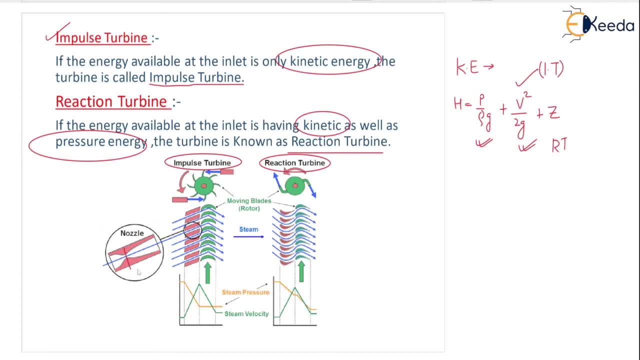 nozzle And this nozzle is, you can see, it is convergent, divergent nozzle And this nozzle will這樣的 nozzle Correct Mach number will be one at the throat. So this nozzle, This nozzle is passing through the stator and then rotor. You can see the 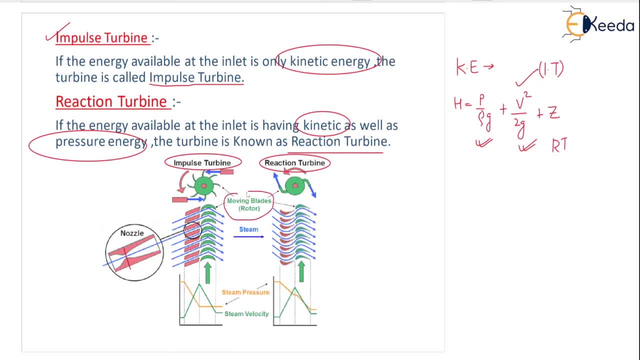 green colour blades, moving blades, also mentioned as rotor, correct In both the case. And red colour is the stator part. Okay, So what happens the first? the liquid or fluid will pass through the stator, then it goes to the rotor. So in in all the cases you can see the same. it is happening that the fluid is passing through the stator And then in the next time when it is moving it will move to the rotor, Then if this case, the nozzle is passing through the stator, then it will change the motive. look for the stator. Do you get the? 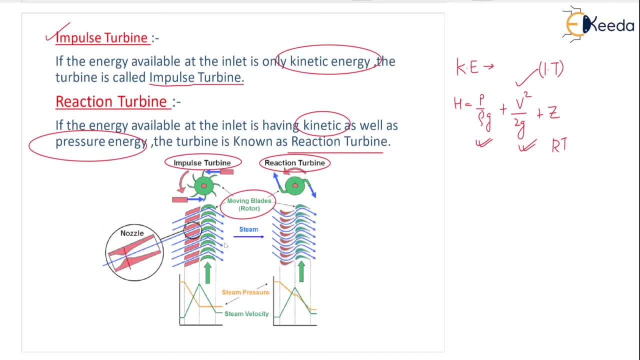 and then it is moving towards the rotor and then coming out and it is steamed and it is steamed. so what happens here? a velocity and pressure diagram is shown here along the stages of the rotor and stator. so velocity, what happens? after entering it with the stator? the velocity increases. you can see the green color. 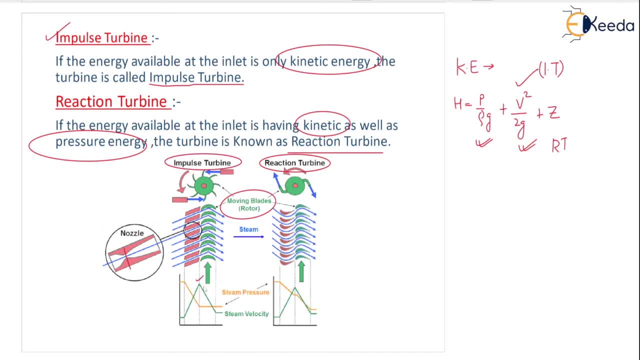 line the velocity increases and in this rotor velocity decreases and almost comes to the same level. so there is very negligible change in the velocity when it comes out of the turbine. okay, that is the conclusion. second thing is pressure. you know that in the turbine pressure always decreases. pressure comes. 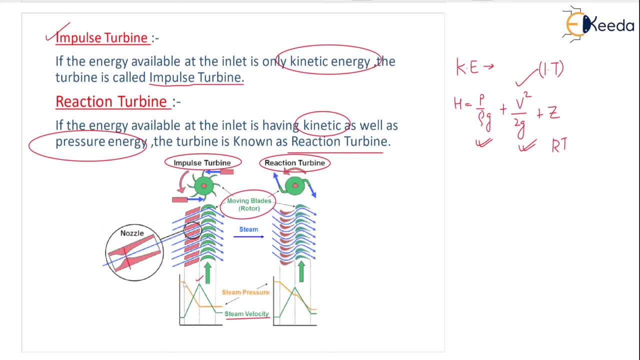 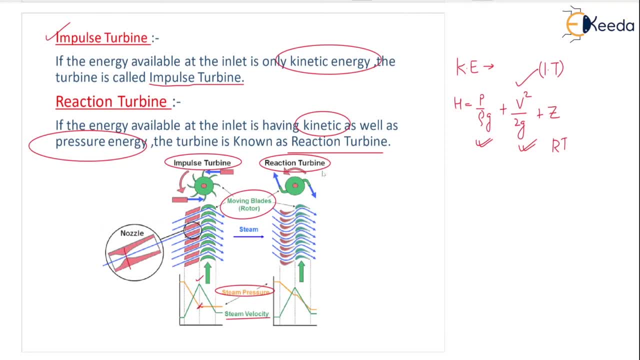 only in the rotor. now coming to reaction turbine, we are going to discuss the same velocity and pressure diagram. so what happens in this reaction turbine? so again, the steam or fluid has to pass first through the stator and then it moves towards the rotor. so you can see the profile difference between the rotor. 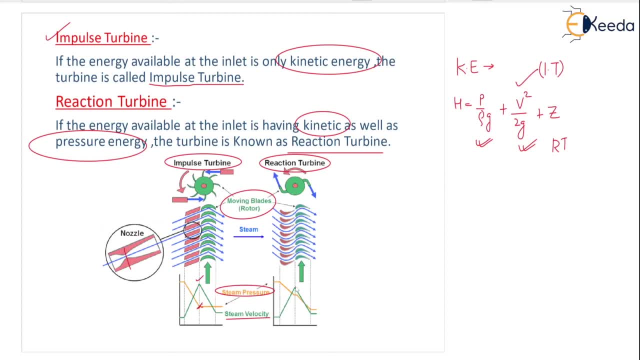 and stator of the impulse turbine and reaction turbine. so same velocity is same. almost here you can see velocity is same. almost here you can see. velocity is increasing from 0.. Turk can see reason one to one and in this simulation and cooled 2017, forgiving the 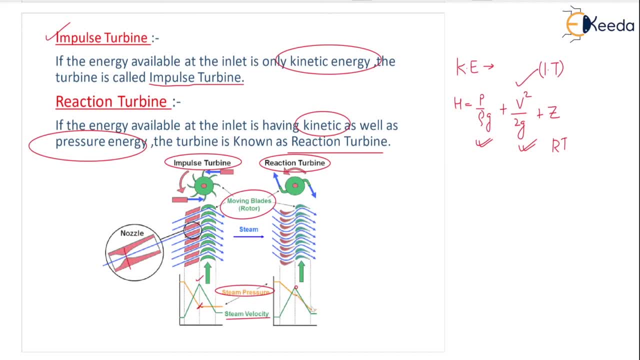 photograph is that this is first increase in the stator and then it decreases in the rotor. first in the stator it is increasing and then decreasing, coming to almost same level, no changing velocity. but if you look into decrement is almost same. if you see these two, it is almost same here. but 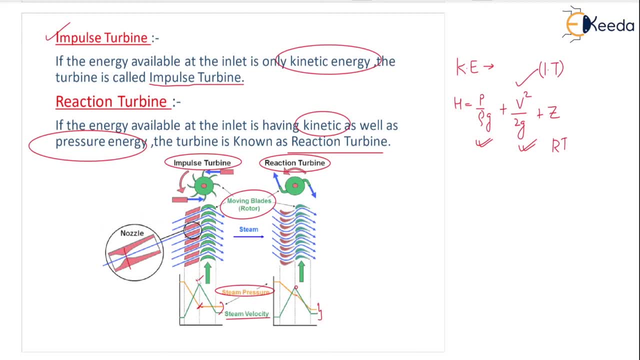 what is the difference between the impulse and reaction turbine? that in the impulse turbine all the pressure decrement is achieved in the stator itself, but in case of reaction turbine we are getting 50% decrement in pressure in the stator and 50% in the rotor. this is one difference. second thing: you can 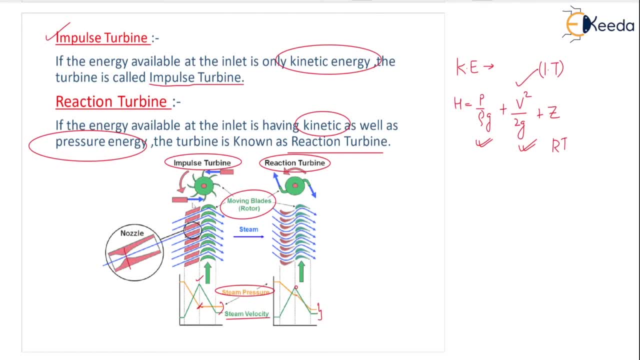 see here impulse turbine, so kinetic energy, jet of water is applying on the blades, so because of that that it is moving. but here you can see, in the reaction turbine jet of water is is in one direction, in this direction. so the reaction, that the turbine reaction can move in this direction, that is your this. 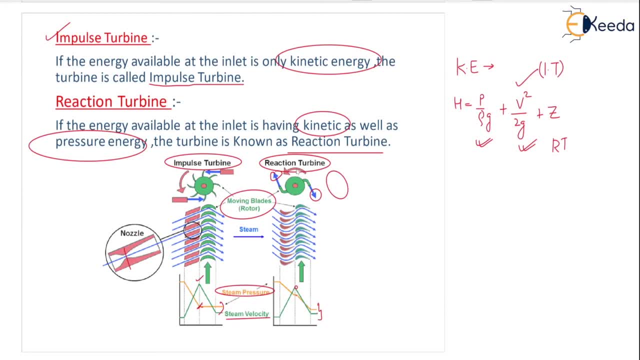 direction is your anticlockwise direction correct. so the velocity as well as you can see, the velocity head of pressure head is applied in case of reaction turbine. so one is this force which is trying to move the turbine in the anticlockwise direction and second one is because of 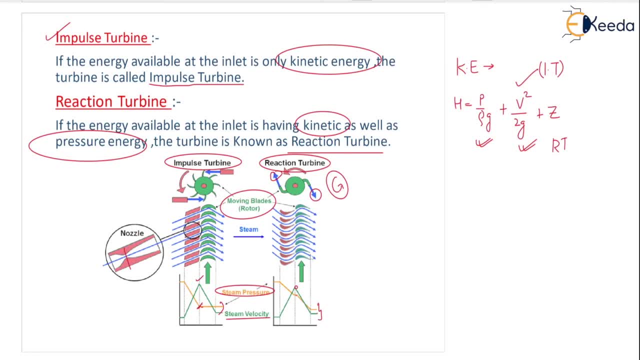 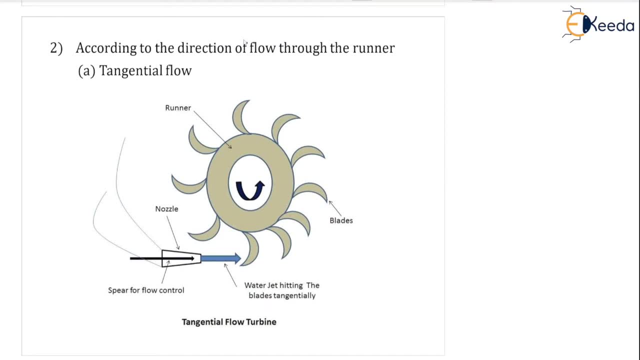 the this velocity jet. let us go into the next slide according to the direction of flow through the runner. direction of flow through the runner: tangential flow. this first one is tangential flow, you can see. so this is the runner. we have already mentioned here, this is the runner, and 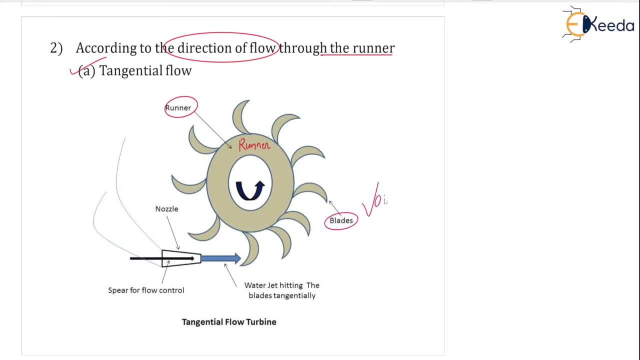 blades, also known as vents and nozzle, and so the direction of water. you can see it is tangential to the runner, or tangent to the runner, so it is called a tangential flow turbine. so you can see it is written here: water jet hitting the blades tangentially and 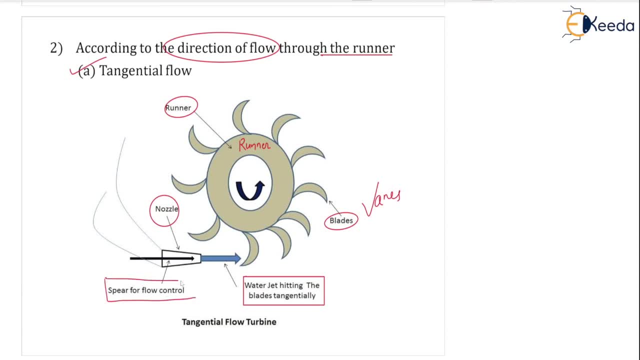 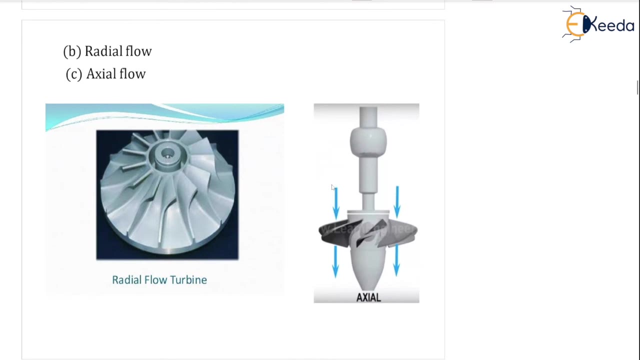 spear for flow control, mass flow rate control. a sphere is there, so it is tangential flow turbine. okay, what is the direction of rotation? nice, nor rotation is anticlockwise. it is mentioned next is depending on the direction of flow. another one is radial flow and axial flow. so you can see the example of radial. 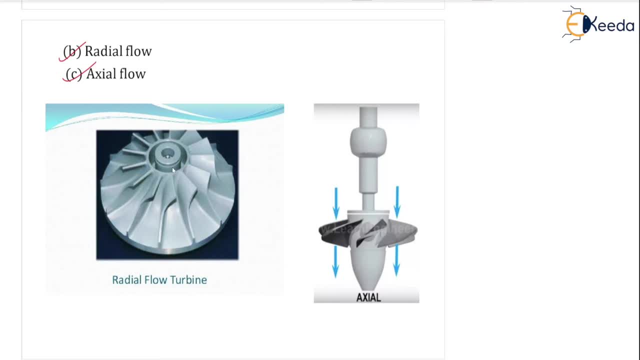 flow turbine, correct. so the movement is along the radius, along the radius you can this path right along the radius, but that is called radial flow turbine. and when the movement of the fluid is along the, or you can say movement to the fluid, is parallel to the axis, it is called 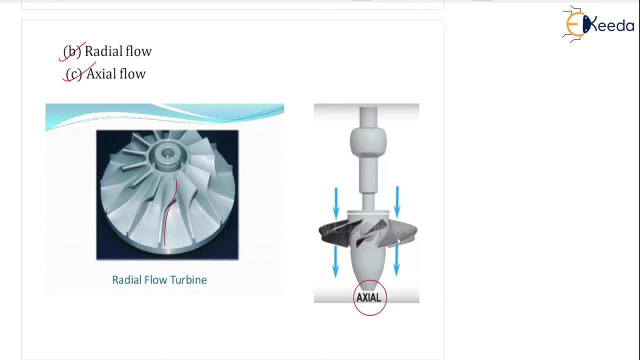 as axial flow turbine We can see. in this case, the direction is parallel to the axis, So this is the axis you can see here. in this case, this is the axis you can see, so it is parallel to the. that's what is called as axial flow turbine. 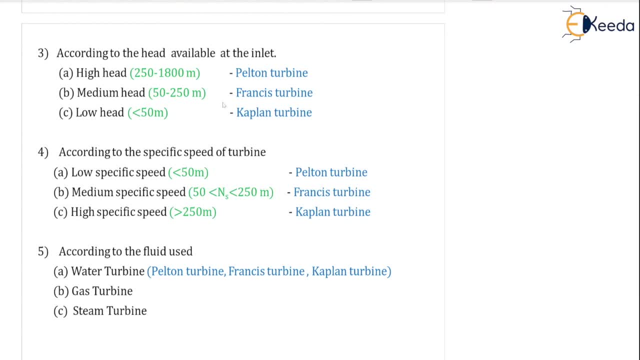 according to the head available at the inlet. this is the third one head available. head means we are talking about the magnitude, magnitude of head, like high head turbine. high head means 250 to 1800 meter. then it is called high head turbine. example is a built-in turbine. second one is medium head: medium. 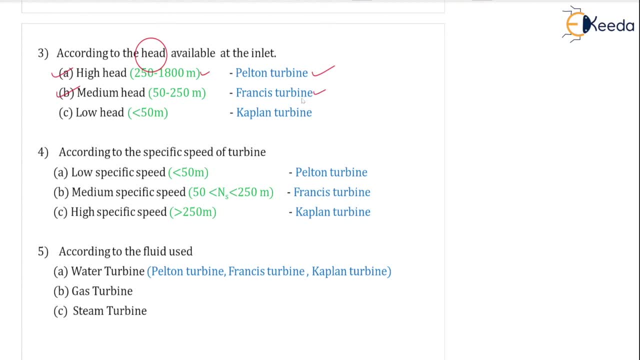 is 52 to 50 Francis turbine, the example. and low head is less than 50 meter and example is Kaplan turbine. so Kaplan turbine is low head, axial flow turbine. Francis turbine is reaction turbine, whereas built-in turbine is impulse turbine. so along with this type of turbine, we should also remember the head available. then 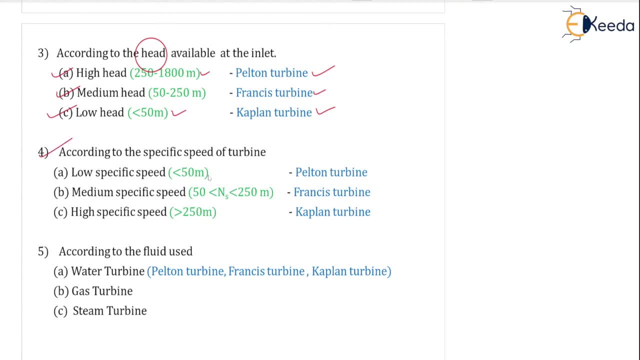 according to the speed of the turbine. we are having low specific speed, less than 50, less than 50 actually. so it is built-in turbine and we do have a specific speed: 50 NS 250, then it is Francis turbine and high speed turbine is your. 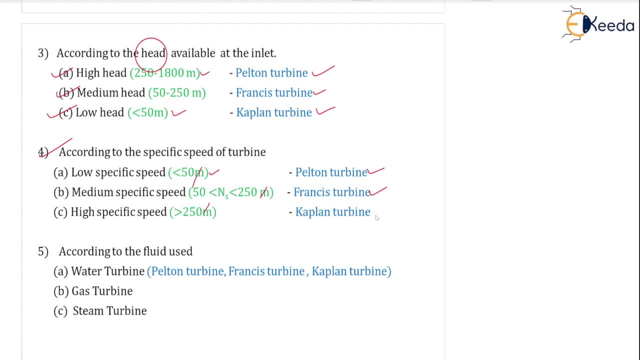 high speed turbine is greater than 250. it is Kaplan turbine. so low specific speed. we are going to see what is specific speed. so your N is your RPM. whenever you are giving some condition to the RPM- normal RPM- it is called as specific speed. that means some specific condition is given to the RPM and